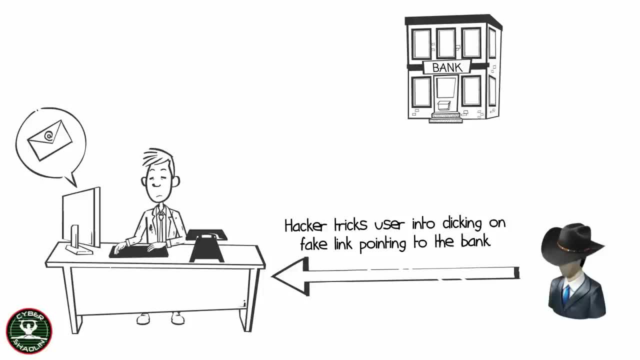 trusted location, but really it connects to your bank. So when the user clicks on the fake link, it uses the previously set session token. The hacker's request is executed and the user's account is hacked. For example, money from the user's account can be transferred to the hacker's account. 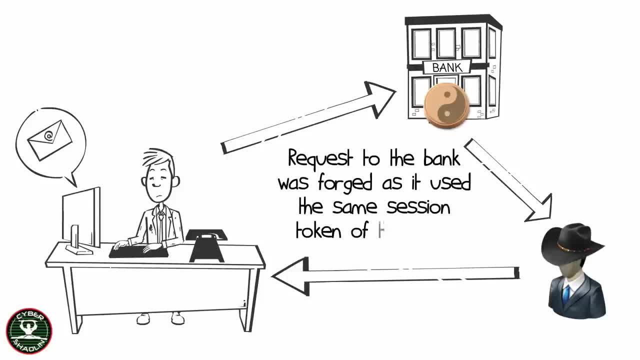 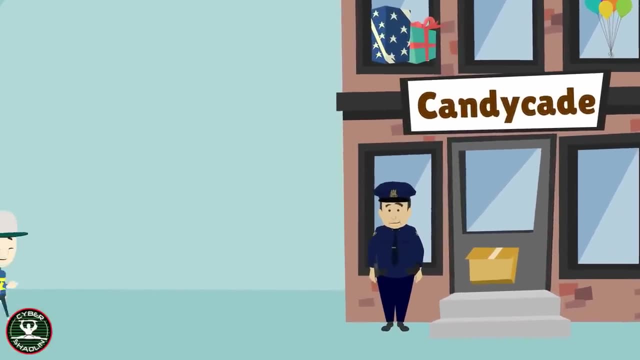 So how did this happen? The hacker's request to the bank was forged, as it used the same session token of the user, which did not require the user to log in again. A simpler way to understand CSRF is as follows: You are invited to a birthday party in a candy shop. 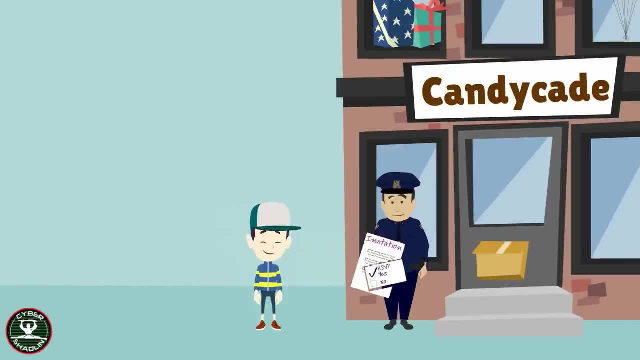 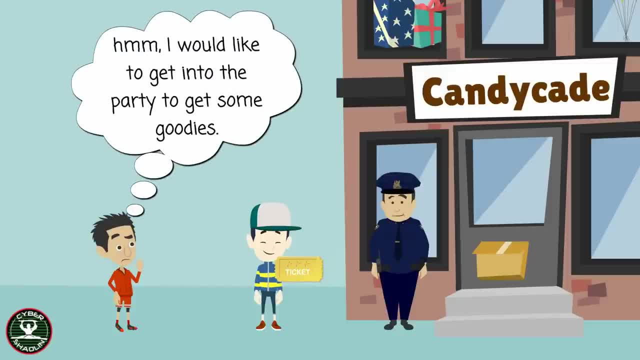 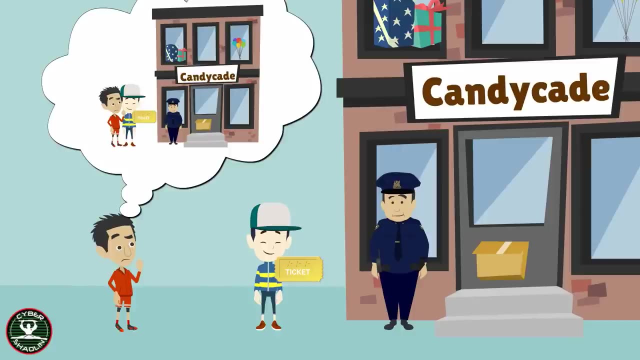 The security guard will check the invitation and give you a message. The security guard is DP, So he thinks to himself: maybe I can trick the kid with the ticket to go in and I can sneak in behind him lines. Hey, buddy, did you know the first 5 kids to the party get a special prize. 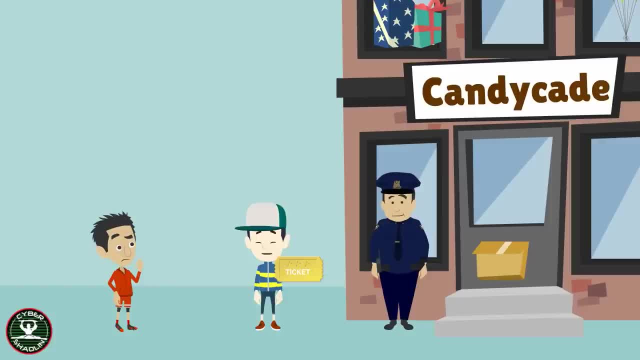 Champion Neon Prime. Wow, I never knew that. Thanks for taking my 만nellobad agent account Thumbs up right. thanks for telling me. so you show your ticket to the security guard and you go on it in. the bad kid sneaks in behind you. 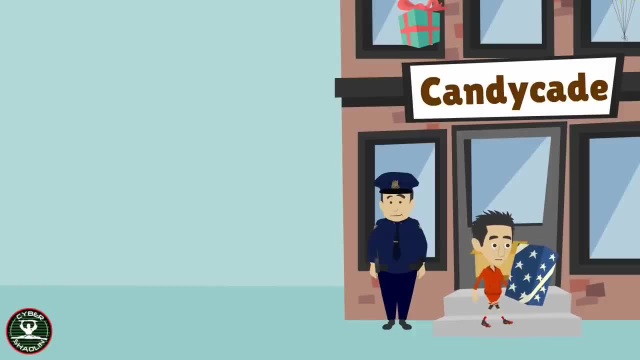 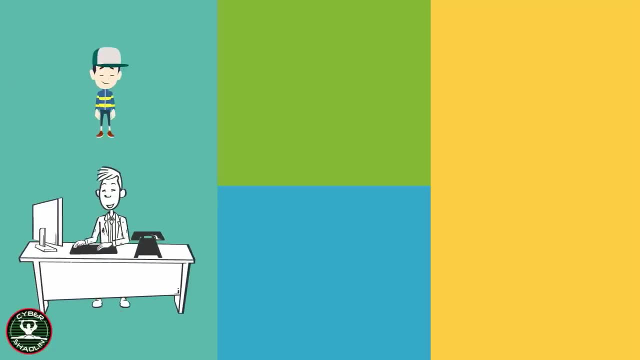 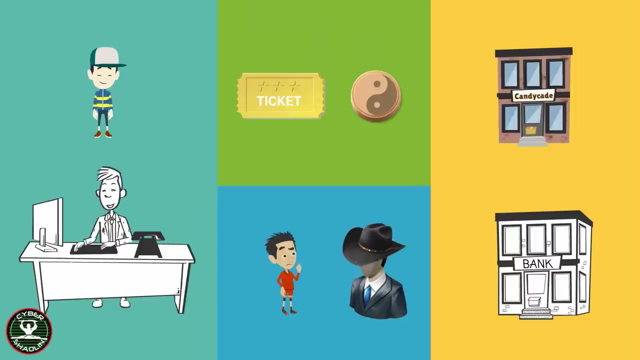 a little while later, the bad kid walks out with a goodie in his hand. so how does this relate to CSRF? the good kid is like the user, the candy shop is like the bank, the bad kid is like the hacker and the ticket is like the session token. 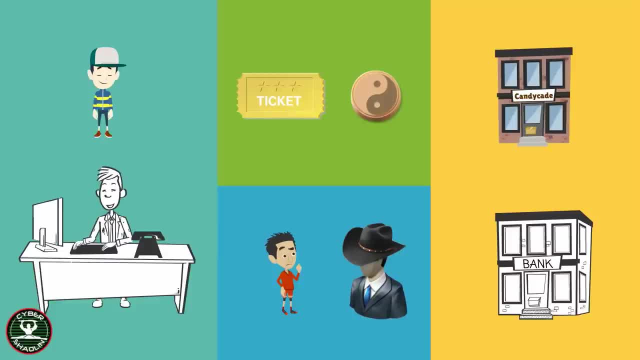 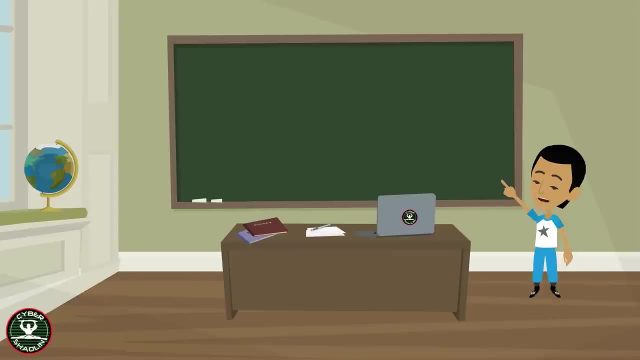 CSRF is possible when a hacker can use established session tokens of the user without any additional verification, just as the bad kid used the good kids ticket to get into the party and get himself a goodie you, in this video you learned about cross-site request forgery and for more.